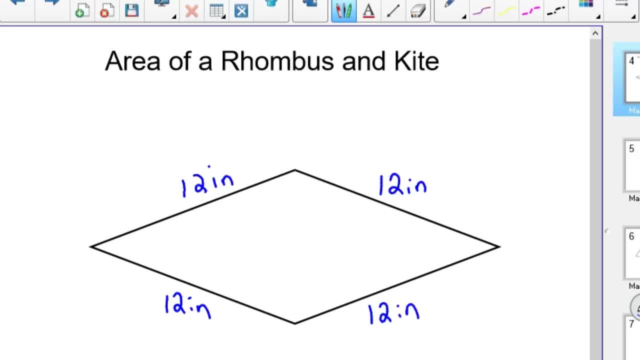 And, as it is, we wouldn't have enough information here to find the area of this, So we'd need one more piece of information, And so typically what they might give you is an angle, Or, in this first case, I'll just give you the length of one of the diagonals. So let's say they gave you a diagonal. See, all those were 12.. Maybe this is 8 inches. 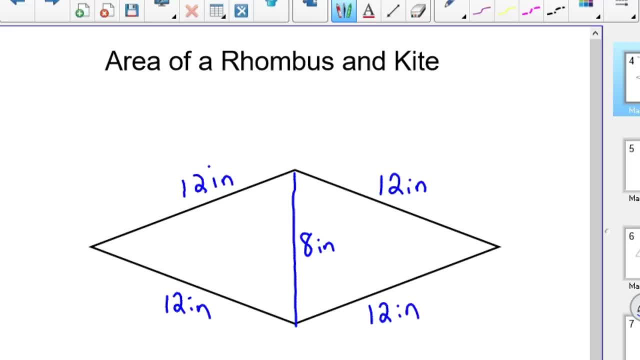 And it's a find the area of this thing. Well, immediately when I drew in that diagonal, you can see it's split into two triangles. So you know, hit pause and see if you can figure this out. What is the area of this rhombus? 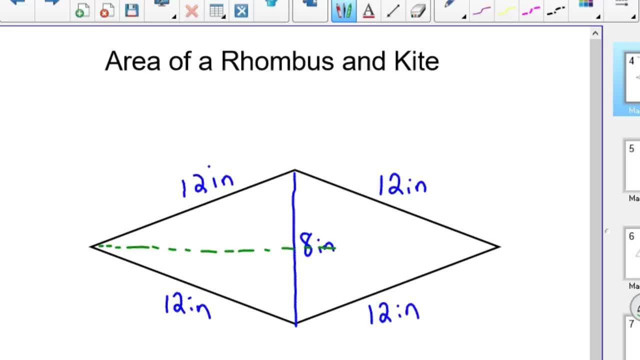 Well, the thing about a rhombus is it splits it up into four. If you draw in your two diagonals, it splits it up into four right triangles that are all equal. So this length here is now four, And we don't know this length. 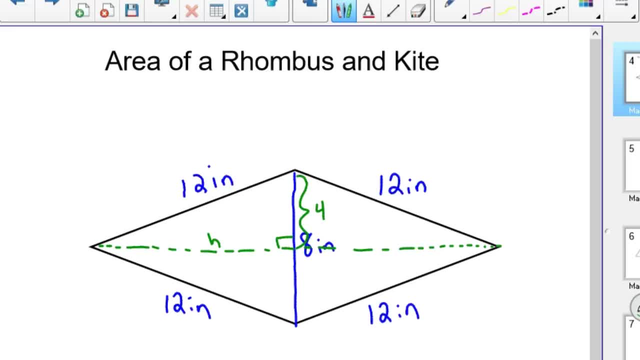 Well, anytime you have a right triangle where you're given two sides, you use Pythagorean Theorem. So 4 squared plus h squared equals 12 squared. So 16 plus h squared equals 144.. I'm not sure why I put it to the fourth power there. 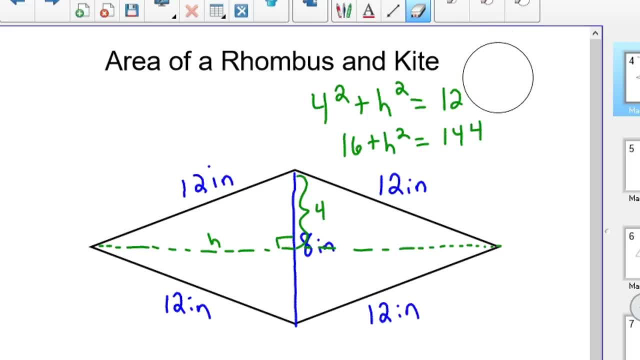 That should be squared. That was weird. Uh uh, maybe too late at night for this video, But anyway, 4 squared plus h squared equals 12 squared, So 4 squared is 16.. 12 squared is 144.. 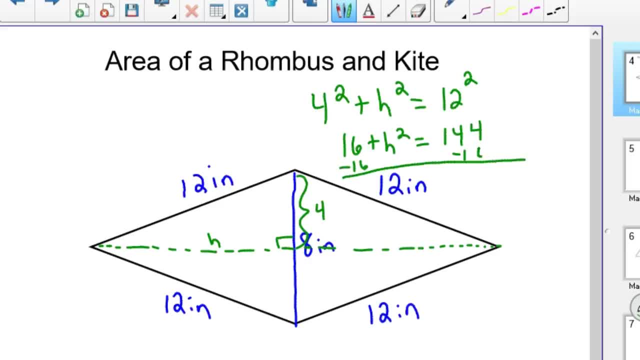 Then you'd subtract the 16 from both sides And h squared equals 128. Then you would, if we want that particular height, you'd take the square root, then Square root of 128. We can break that down. Square root of 128. We can break that down. 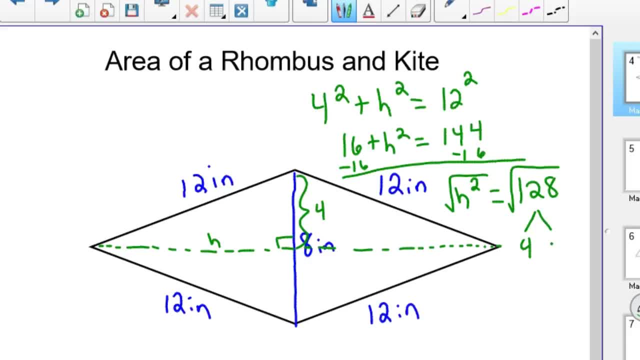 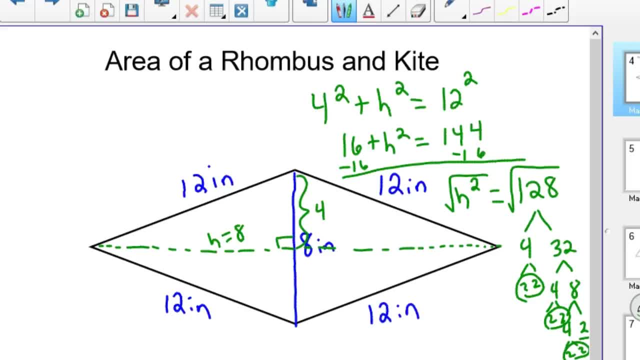 can't change anything- can't change anything- so the height of this thing is 8 root 2. now it's also- you could have just found- the square root of 128, which you know it's 121 is. square root of 121 is 11. so 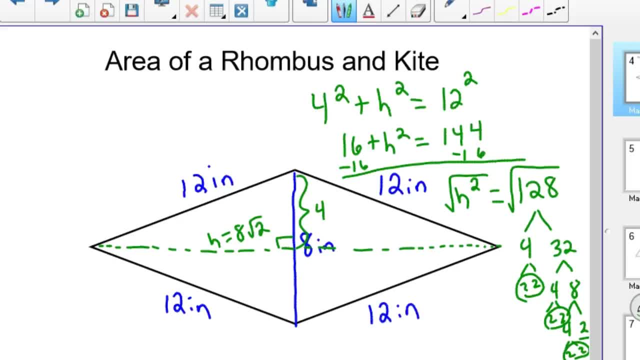 this is slightly more than 11 and less than 12, obviously, but if you're doing a college entrance exam, they want the exact value. they want this 8 root 2, so there's lots of ways to figure this out. now you could find the area of each of. 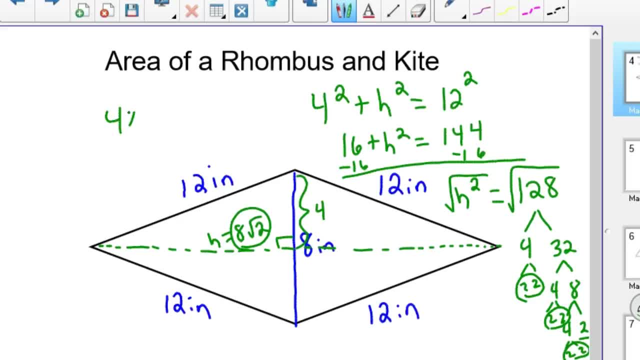 the four triangles. so you could take 4 times 8 root 2, which is base times height, and then divide that by 2, but then you that would give you the area of one of these. then you'd have to take that times 4, because there's four of. 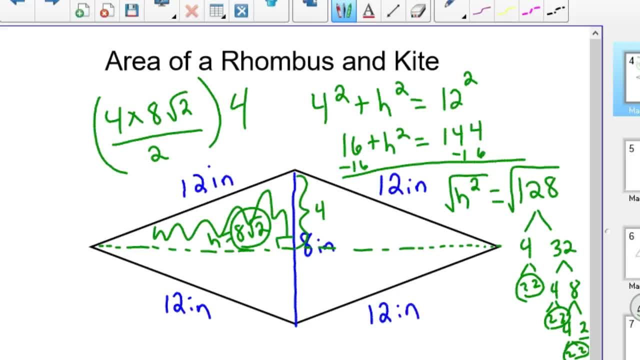 those triangles. so if you went ahead and finished that, 8 times 4, you know, divided by 2 that's 8, that's 16 root 2, but it's still times 4. so each triangle, each of the right triangles, is 16 root 2, but you still have to take 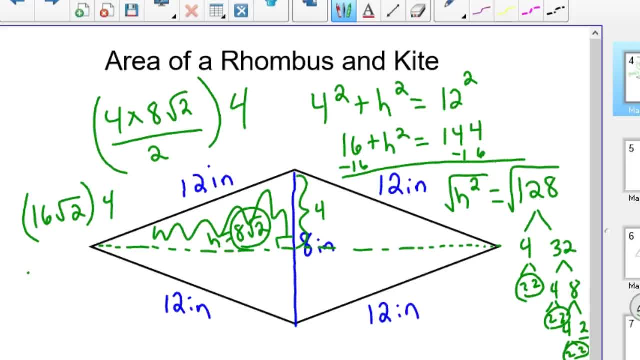 that times 4, which gives you an answer of 64 root 2, because 16 times 4 is 64. so that's the area of this particular rhombus. so that's the area of this particular rhombus. so that's one type of these problems. you could also have a kite, and I don't have. 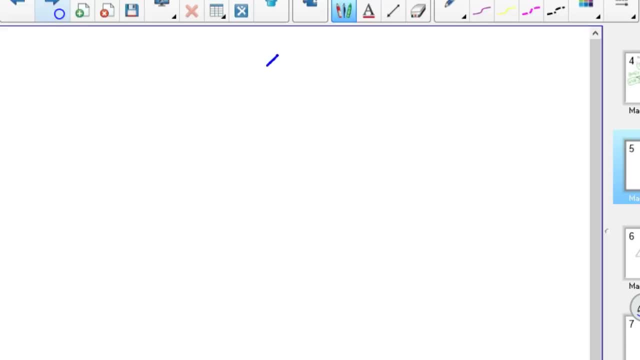 a nice picture of a kite, but in mathematics a kite means you have adjacent sides that are congruent, but just two sets, and so there's what it looks like. you know, this might be 12 and this might be 12, so that makes this maybe 20 and this 20, so those are the adjacent. 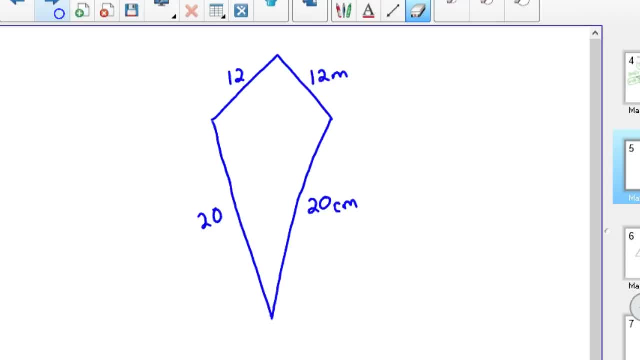 sides that are congruent, kind of generally what you think of as a kite shape. when I was a kid I was flew bat kites so it wouldn't look the same. I would have always thought of a bat instead of instead of this when I hear: So you've seen the word kite, but in mathematics this is the shape of a kite generally. 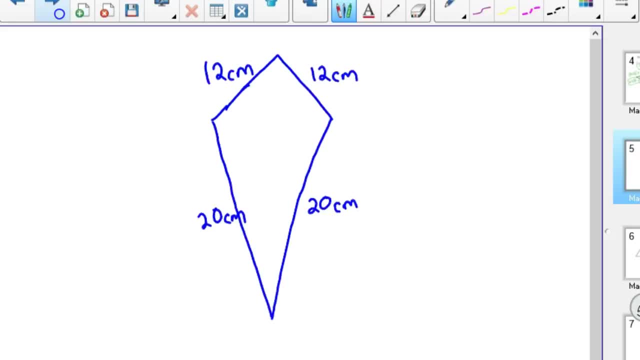 Now again, there's not really enough information to solve this thing without one more piece, And so usually you have a diagonal, And again what you end up with is two right triangles on the top that are equal, two right triangles on the bottom that are equal. 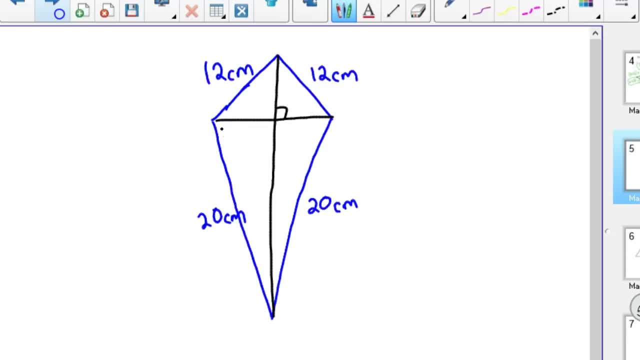 And so they might give you one whole length of a side here, this whole diagonal, Maybe, that's. we'll go with eight again, And so pause the video and see if you can find the area of that thing. So give it a shot. 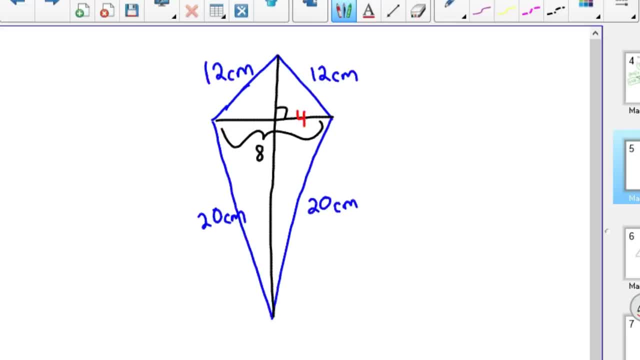 Now, I know so that this one now is four, and this is four because we split that exactly in half. They're perpendicular bisectors of each other, those two black diagonals, And we want to know this height here and this height here. 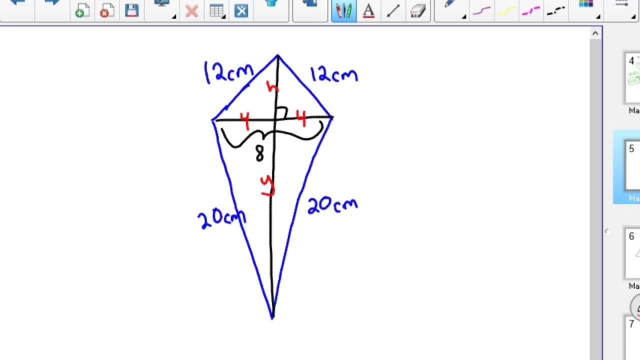 which I'll call y, just so it's a different variable. So, and we have right triangles everywhere, so you can do Pythagorean Theorem. So four squared plus h squared equals 12 squared. That gives you the height of the top one. 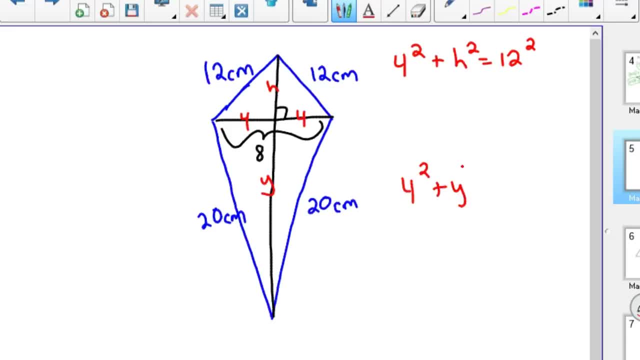 The bottom one would be the height of the top one. The bottom one would be four squared plus y squared equals 20 squared And you solve both of those. And we already found this h here. in the last video We had the similar problem. 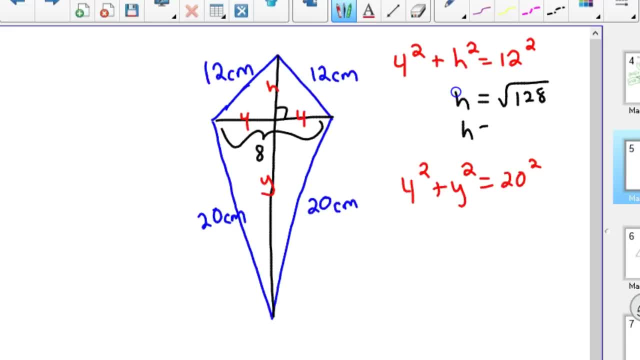 So h is the square root of 128, which is also equal to- I think it was- 16 root 2.. Let me double check that. All right, Oh, 8 root 2.. Pardon me, I just remembered it wrong. 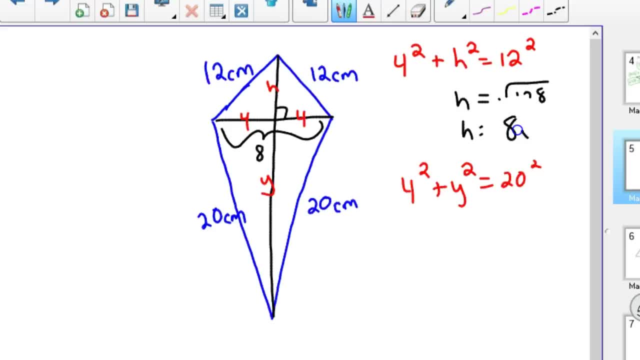 I didn't want to go through all that work again, So that's 8 root 2.. And the bottom one. we haven't done that one yet, so we'll go ahead and finish it. 16 plus y squared equals 400.. 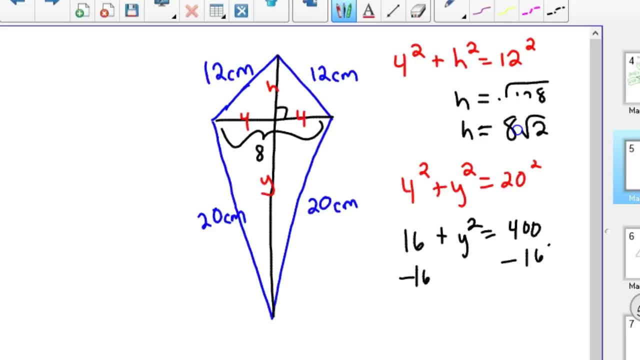 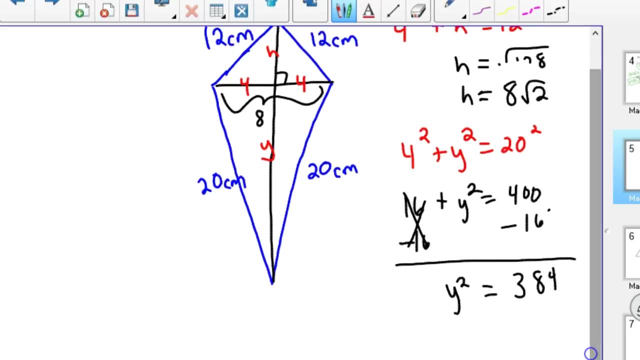 You subtract the 16 off, And so y squared equals, because those cross- I haven't been really doing that- 400 minus 16 is 384.. And so you take the root of that, Take the root of that, And again we have to get that. 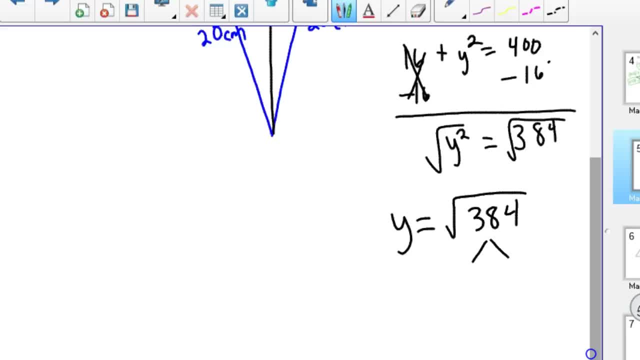 We have to get that square root so we can get the exact value. So if we break that down, we can take this into 4.. And then that would be 96. We can break that down. We can break the 96 down into 4 and 24.. 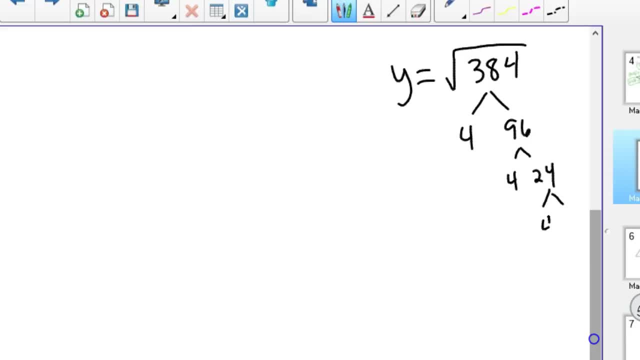 We'll keep going down. 24 breaks into 4 and 6.. And 4 is 2 and 2.. 6 is 2 and 3.. 4 is 2 and 2.. 4 is 2 and 2.. 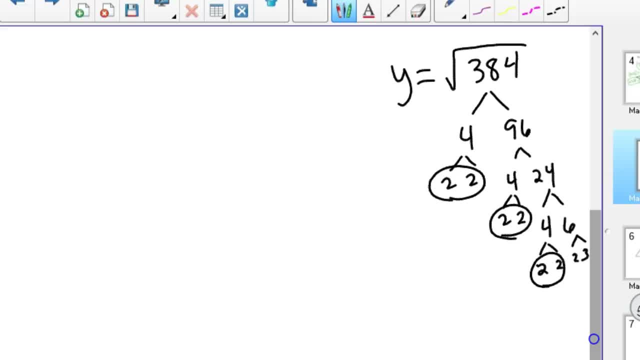 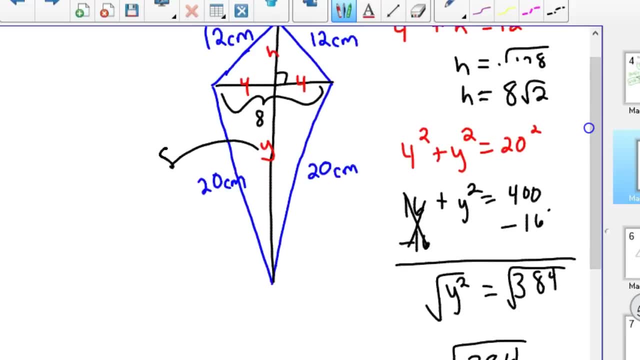 So there's a pair, There's a pair, There's a pair, So that would be 8 root 6. So that's y And h was 8 root 2.. So, in terms of finding the area of these, you could find the area of this top triangle. 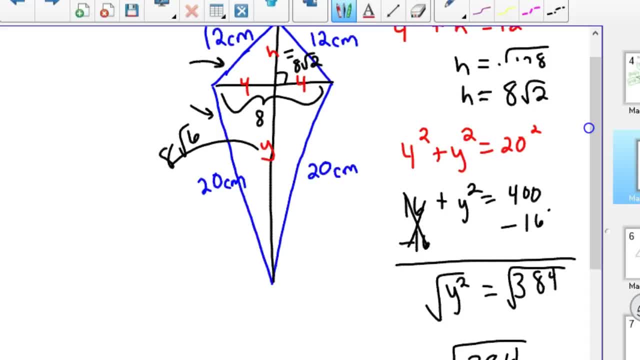 times the area of this bottom triangle. So the top one would be 8 root 2 times your base, Which was 8 divided by 2.. And the area of this bottom triangle again 8 root 6 for your height. 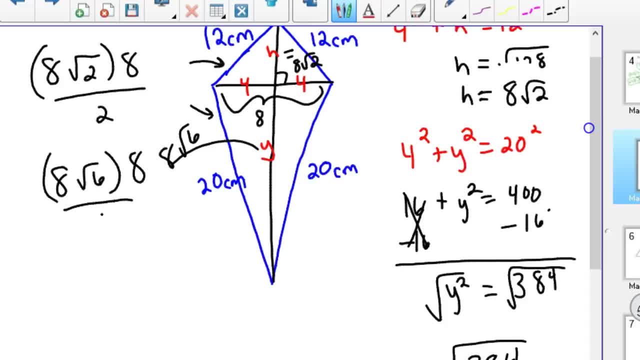 Times your base of 8 divided by 2.. And so you'd be looking at this top one here: 64 root 2 divided by 2, which would be just 8 times 4,, which is 32 root 2..